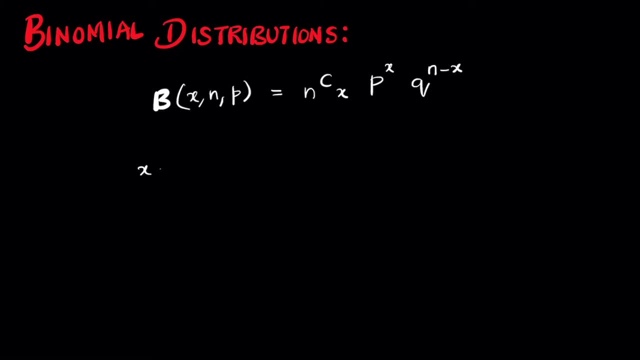 x. So here x represents the desired event, n represents the total number of trials and finally, p represents the probability of success in one trial And q represents the probability of failure. So this is the difference in all of these values. So why do we use binomial distribution? So binomial distribution, also called the, 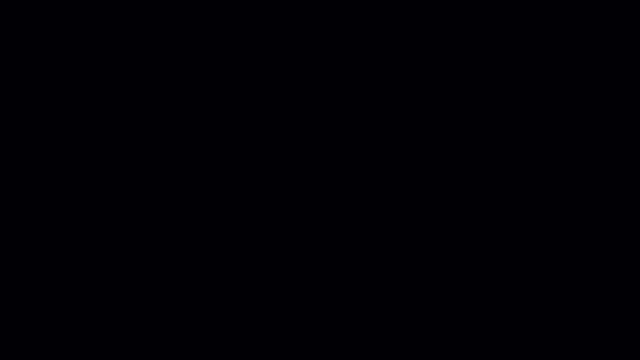 Bernoulli distribution. So is a common distribution where if you have repetitive events and we want to find the probability of success in repetitive events, then we use binomial distribution. So we use binomial distribution when you have repetitive events, So that 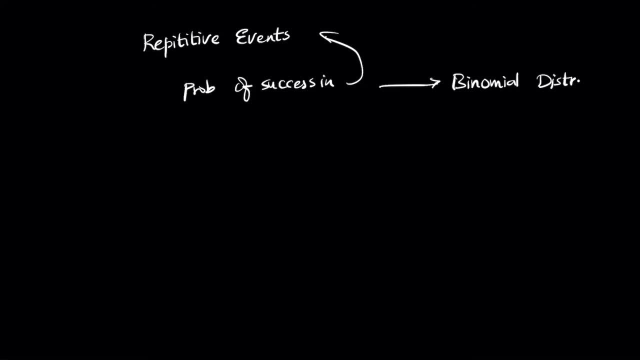 is the case where you would generally use binomial distributions. Now this brings us to the question of what type of cases vary. Where we would, where you would, use repetitive binomial distribution is where, if you have a sample of n independent trials, So where there are only two outcomes, So the outcomes 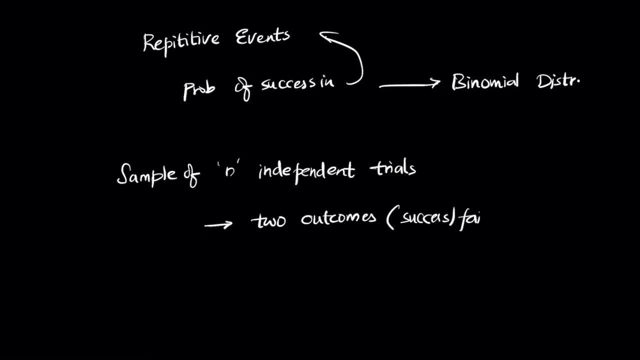 are either a success or failure, Right. So the probability, The probability of success in each trial, we call it p. So p represents the probability of success in each trial, Q represents the probability of failure in each trial. So 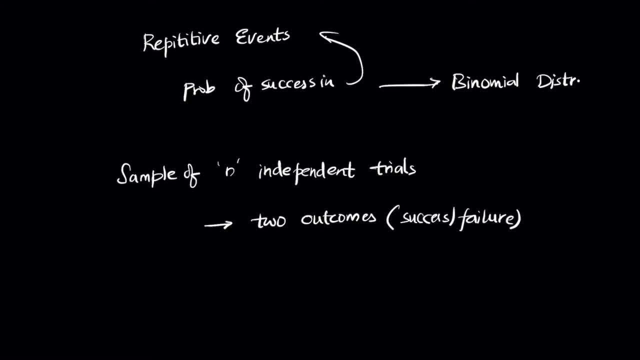 when we consider the idea here is that whenever you consider repetitive events that are independent from each other, So each trial is one event, So you are repeating the same event, which means that you are repeating the same. For example, if you toss a coin, five times what. 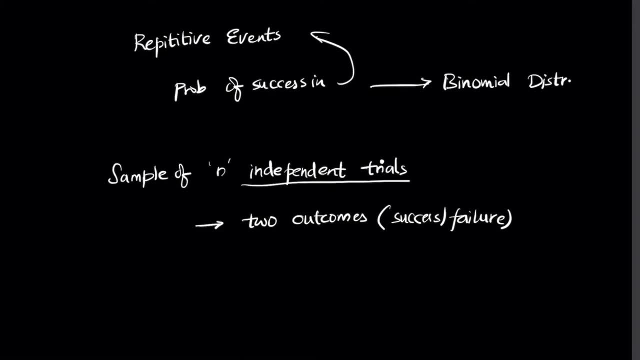 are the chances that you get three heads. So in that case, for example, let us take a problem of five coins and what are the chances of getting three heads? So n here represents five, x here represents three. So p here represents the probability. 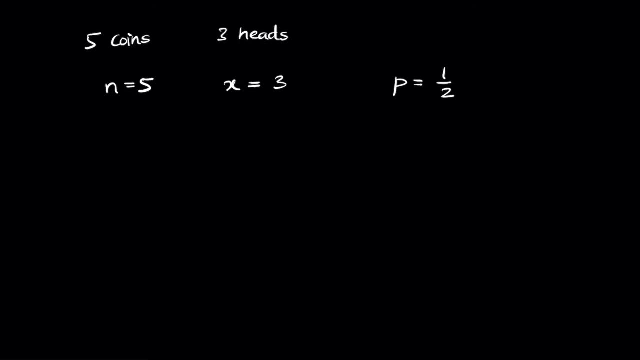 of a head one. you throw once. So when you throw once, the probability of a head is one by two. The probability of failure is also one by two. So these are the data points that you need And you want to know whether you fit is exactly. so there are three words. 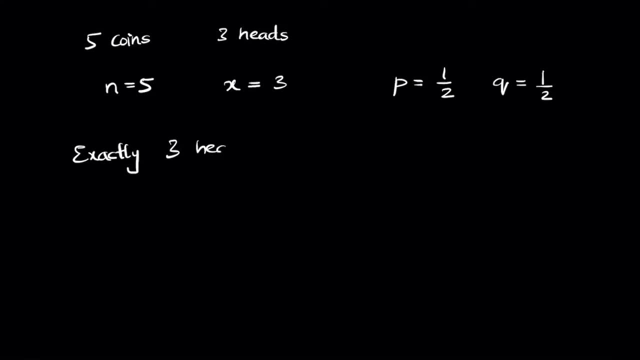 that you will generally see Exactly there. So if you were to add the probability of exactly 3 heads, for example, if it's exactly 3 heads, you will find the probability of x equal to 3 if it is at least 3 heads. it means that you have to have a minimum of 3 heads, which means that 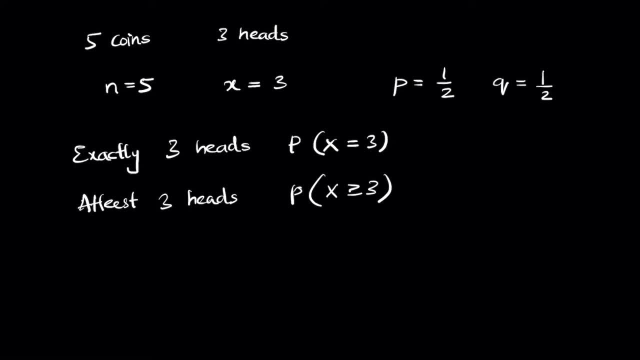 it can be x. x is greater than or equal to 3. next, at most 3 heads is the probability of x less than or equal to 3, right? so at most 3 heads and at least 3 heads. so this is how you see the term. 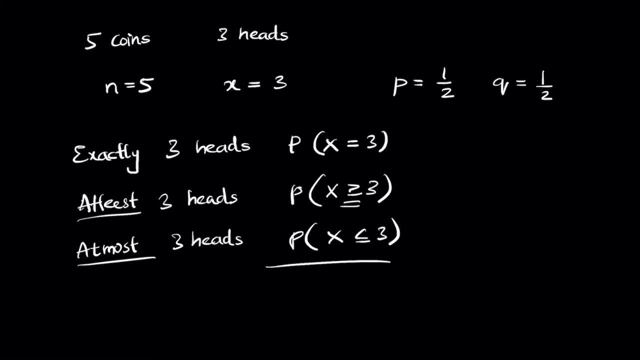 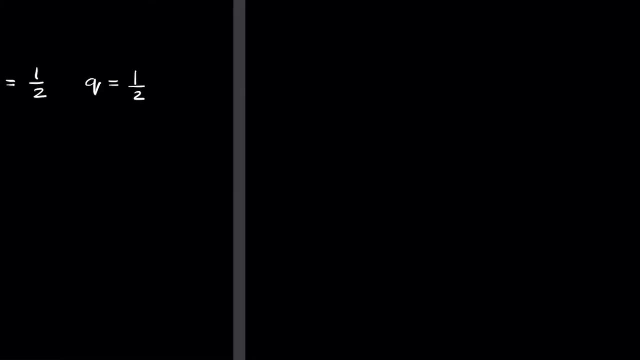 at least at most. so at least represents greater than or equal to. so at least represents greater than or equal to, and at most represents less than or equal to. so these are the three words to remember when you are doing binomial distribution problems. so let's take an example problem and see. 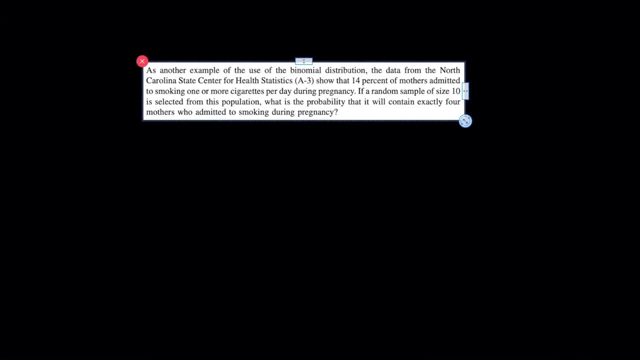 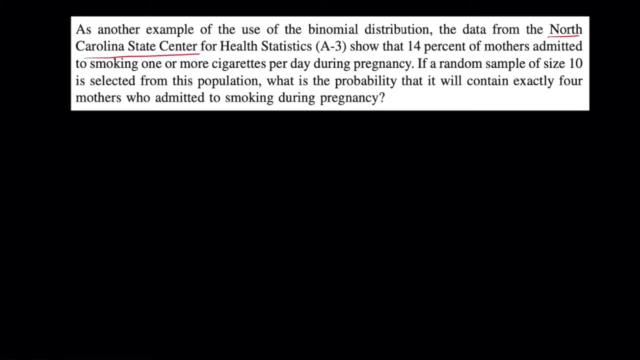 how you can solve the problem. so we have a problem here. so it says that the data from north carolina state center for health statistics shows that 14 percent of mothers admitted to smoking one or more cigarettes during the during pregnancy. if a random sample of size 10 is selected from this population, 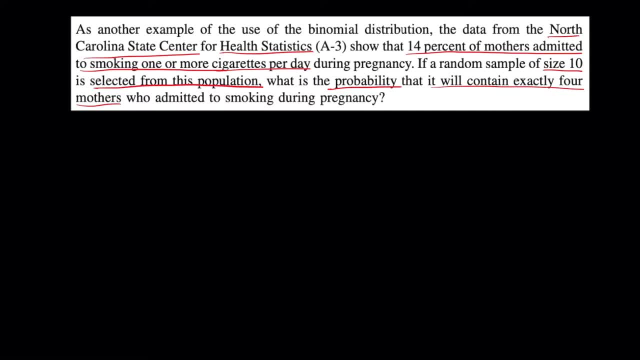 what is the probability that it will contain exactly four mothers who admitted to smoking during pregnancy. so here the total number of trials is the total number of women who are smoking: n equal to n. population of the sample: n equal to 10. out of that x, here is exactly 4. remember the term? exactly 4 here. 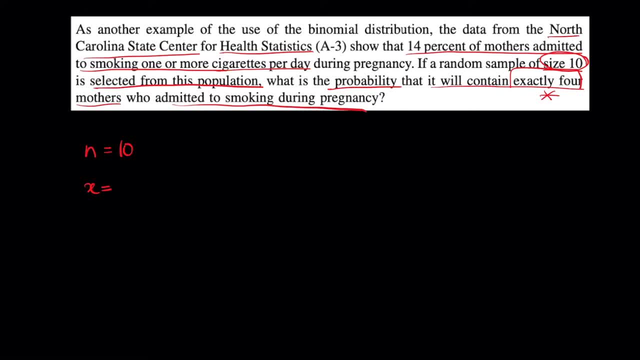 represents that there are only four of them. so out of that there is four of them. x is 4. next is they are asking us to find the probability is given, so the probability is 14 percent. so if the probability is 14 percent, how would you get the value? p becomes 0.14 or 14 by 100? 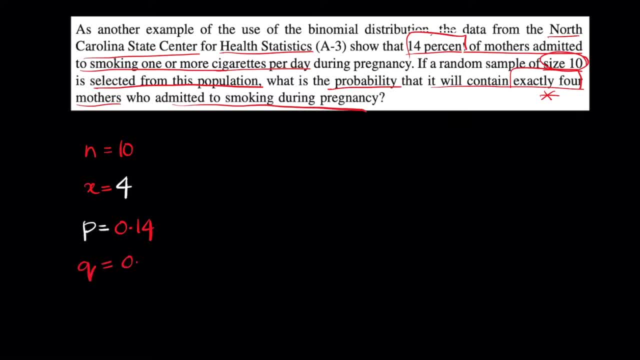 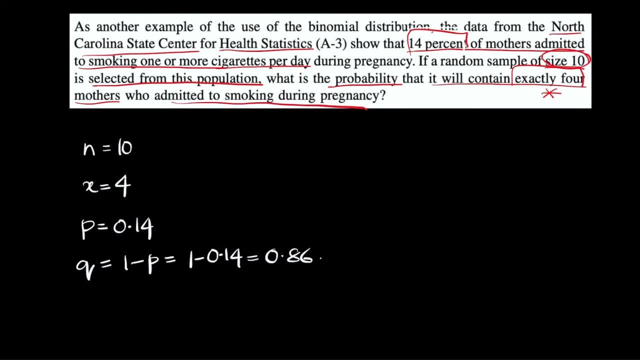 and q becomes 0.14, 0 point. so q is basically 1 minus p, so 1 minus 0.14, so which is 0.86. so these are the probabilities that we have p and q. so the next one we want to know is: we have all? 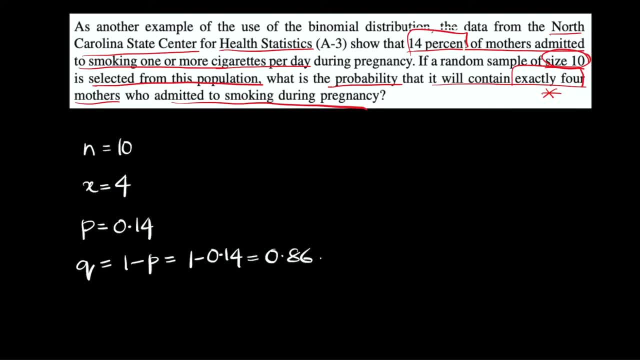 the values, so the probability that they are asking for is exactly 4, so meaning that we are finding probability of p of x equal to 4, so which is going to be binomial of x comma, n comma, p, so that is binomial of x is 4 comma, 10 comma, p is 0.14, so which is going to be n, c, x, p to the power x. 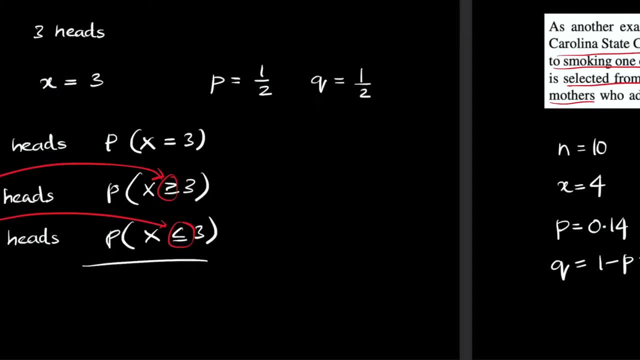 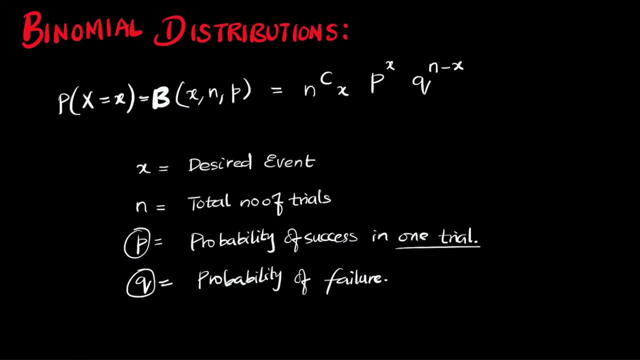 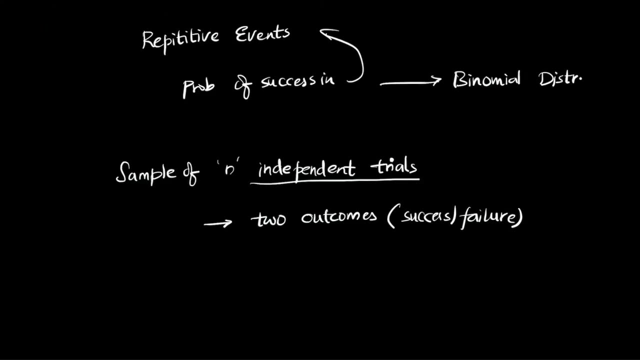 and q to the power n minus x. so remember: the formula here actually represents the probability of one event: x equal to x. all right, so this is the probability of just one event and that is the probability that we are trying to find. now let us try and find the probability. 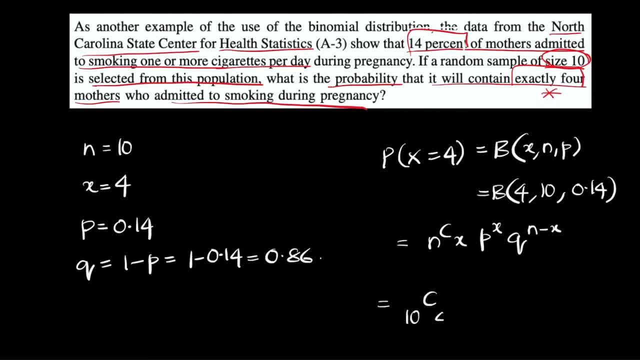 so n here represents 10. so 10 c 4. p to the power x is 0.14 to the power x here is 4, and q is 0.86 to the power 10 minus 4, so that is 10 c 4. 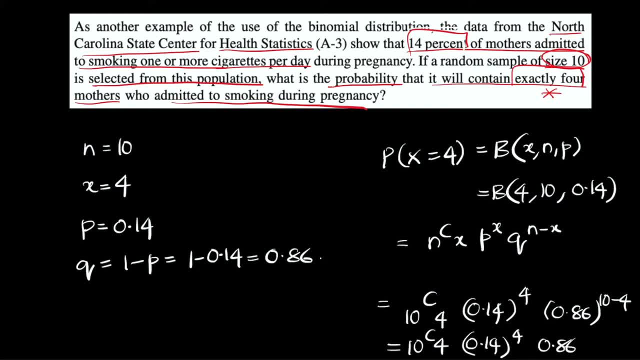 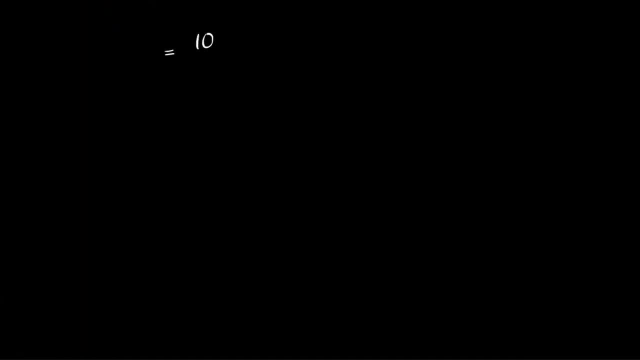 0.14: 0.14 to the power 4 and 0.86 to the power 6.. So now try to find the answer. So use a calculator and try to find the answer. So when you want to find the value here, so remember that this is 10. 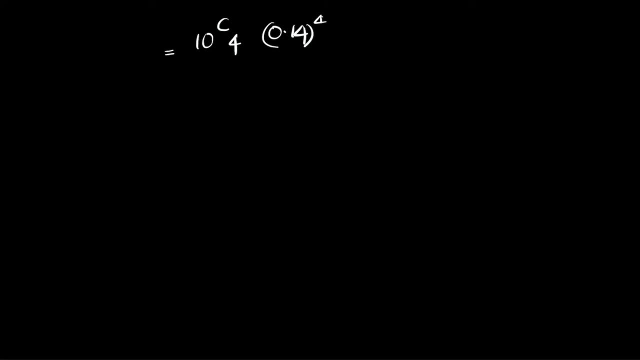 C 4, 0.14 to the power 4 and 0.86 to the power 6.. So 10 C 4 is 10 times. So we can also write it as 10: 4, 0.14 to the power 4 and 0.86 to the power 6.. So how would you write 10: 4 now? So? 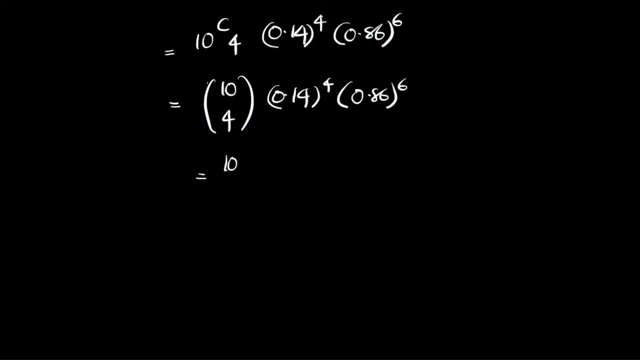 write 10 in reverse, 4 times. So what factorial values? 4 of them. So that is 10 times 9 times 8 times 7, over 4 times 3 times 2 times 1 times 0.14 to the power 4 and 0.86 to the power 6.. 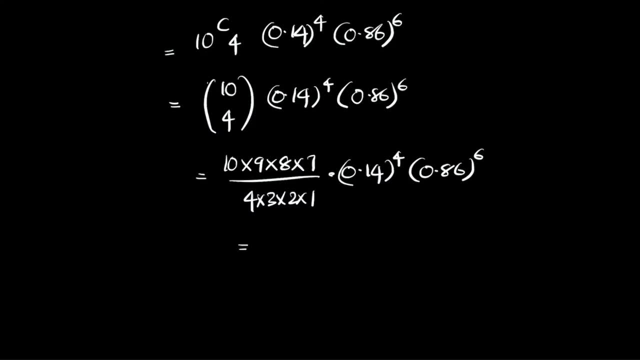 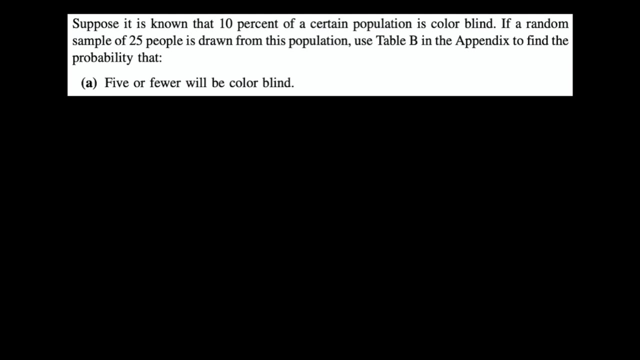 So if you use a calculator and calculate the value, the final answer will be 0.0326.. So this is the probability of x equal to 4.. So this is how you find the probability of the value. So let us try another problem. 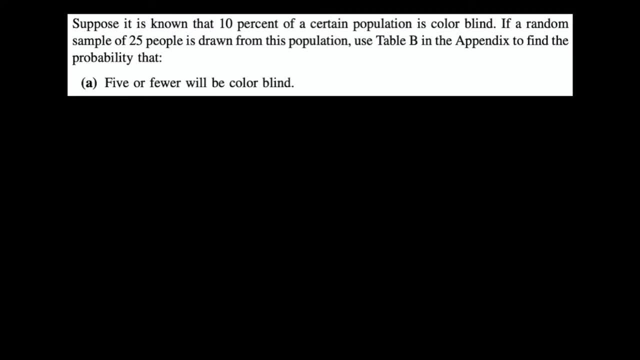 In this they have asked us that. suppose it is known that 10 percent of a certain population is colorblind. If a random sample of 25 people is drawn from this population, find the probability that 5 or fewer will be colorblind Now. so notice that they have. 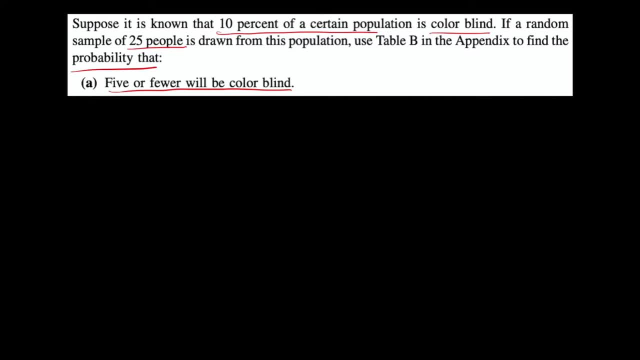 from the total we have. we are taking it out from 25 people. So how do you calculate this now? So this becomes 25.. So they are asking you for 5 or fewer will be colorblind, So 5 or fewer is. 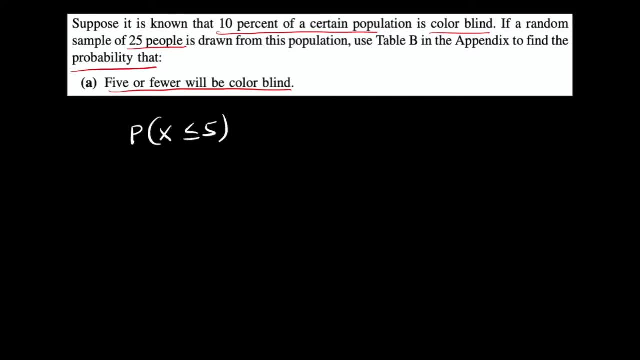 going to be 25.. So this is going to be 25.. So this is going to be 25.. So this is going to be less than or equal to 5.. So how do you calculate p of x less than or equal to 5?? So you can calculate it with 1.. 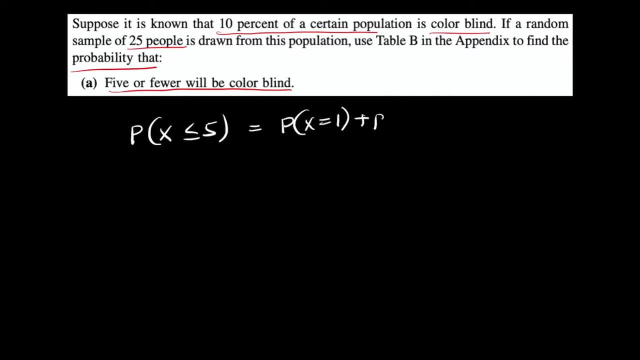 So p of x equal to 1, plus p of x equal to 2, plus p of x equal to 3, plus p of x equal to 4, plus p of x equal to 5.. So, which means that for each of them you will have to calculate: 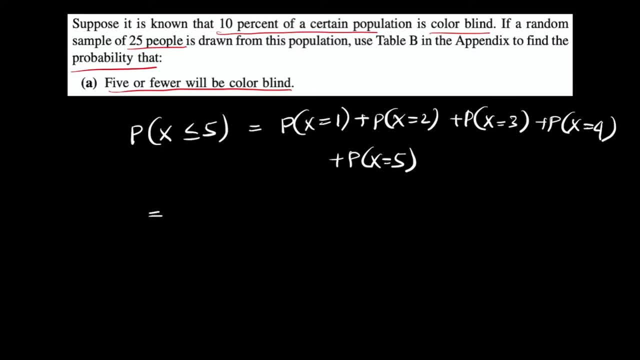 individual binomial probabilities. So to make it easier, we use tables to calculate these values. so it makes it easier to draw the problem. so let me write down the data first, the data is 10, percent is 0.1 and the sample is n is 25. and finally you. 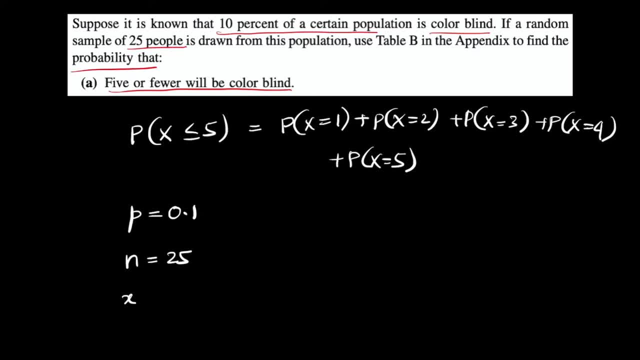 have the x value which is given for each of these problems. so x is 1 comma 2 comma 3 comma 4 comma 5. so to make it easier, what we can do is we can take a table and using that table you can calculate the values. so for our understanding, let's write down the actual formula again. 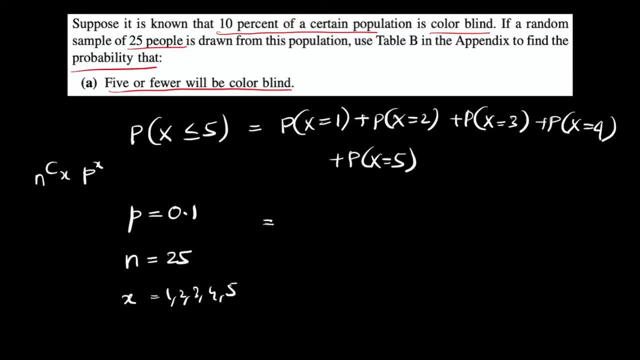 remember the formula is n, c, x, e to the power, x, q to the power, n minus x, so n here is 25 c. 1, p is 0.1 to the power, 1, so q here represents 1 minus p, which is going to be 0.9, 0.9 to the power. 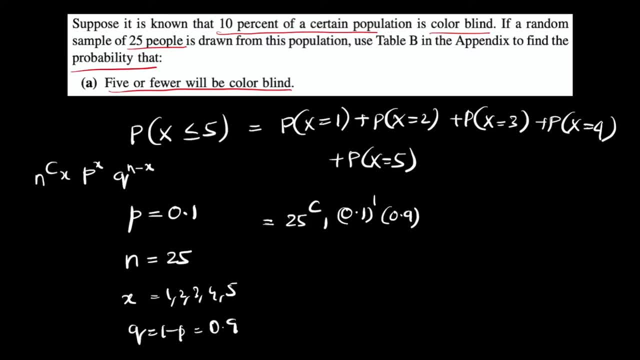 10 minus, so 25 minus 1 plus. next you have 25 c 2, 0.1 to the power, 2, 0.9 to the power, 25 minus 2 plus, and so on until the last one, which is 25 c 5, 0.1 to the power 5 and 0.9 to the power- 25 minus 5. now this seems. 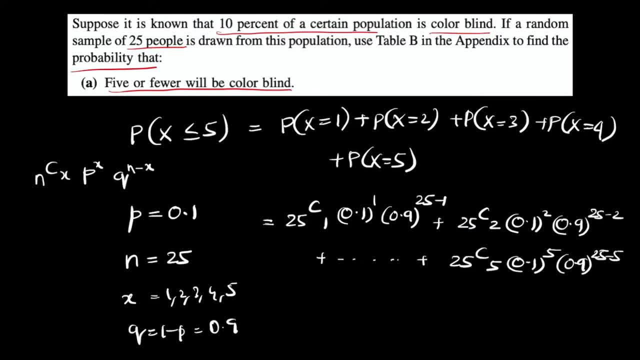 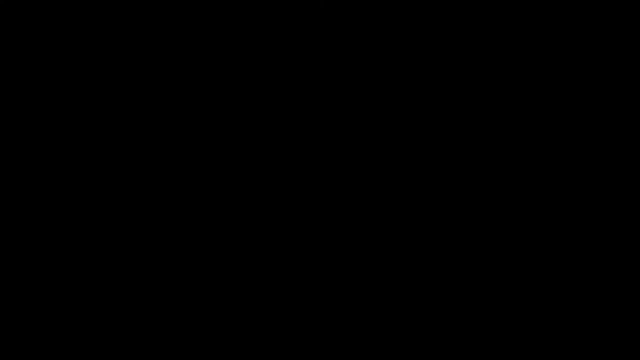 really big to calculate on john in general. so, to make it easier, what we can do is we can use a table. so let me show you how to do that. so let me show you how to do that. so let me show you how the table works. so let me show you how the table works. so this is a part of the table that. 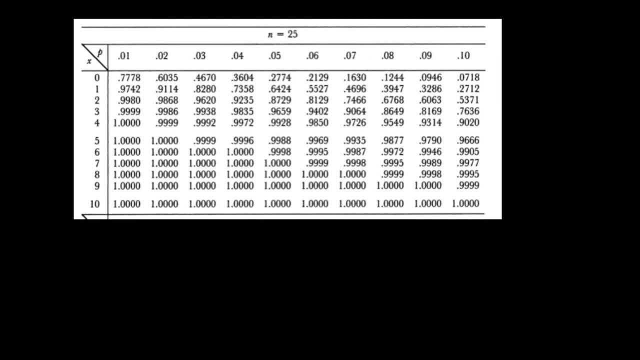 i have taken for our reference. so i'll be attaching this table on canvas so you can find it on canvas for your reference. now, remember that we are taking n equal to 25, so that is our n equal to 25, and the p value is 0.1 and the x value we want is from 1 to 5, right? so let me show you how the table. 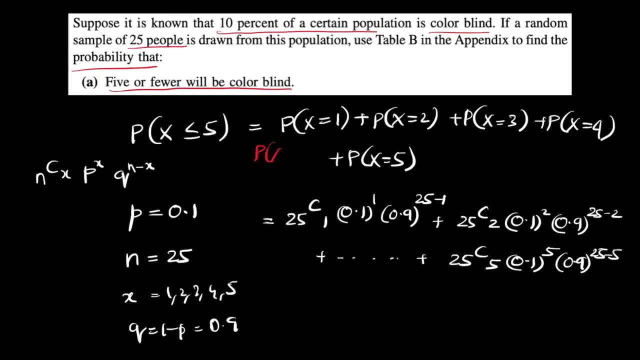 works. so one thing that we also forgot here is the p of x equal to 0, so notice that that also counts as well. so we have to write 25 c 0, 0.1 to the power 0 and 0.9 to the power 25 minus 0. 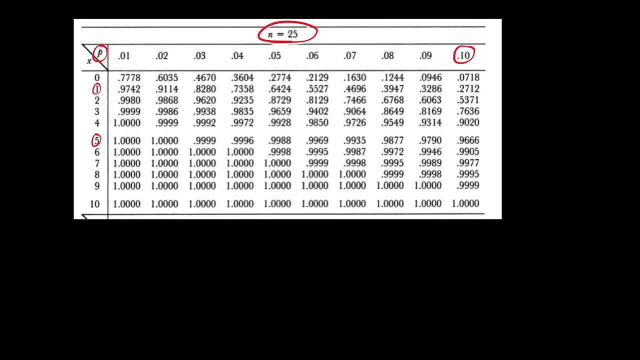 that also counts in as well. so what are the values that we have then? so that is 0.0718, 0.2712, 0.5132, and all of them notice that the values here are given in such a way that when you take for 5, it actually takes. 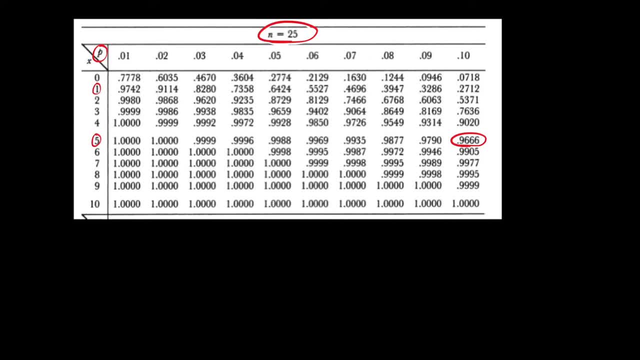 in everything, the sum of from 1 to 5. so the value that is represented here is p of x less than or equal to 5. so that value here is 0.9666. so that is your answer for your problem. so this is the. 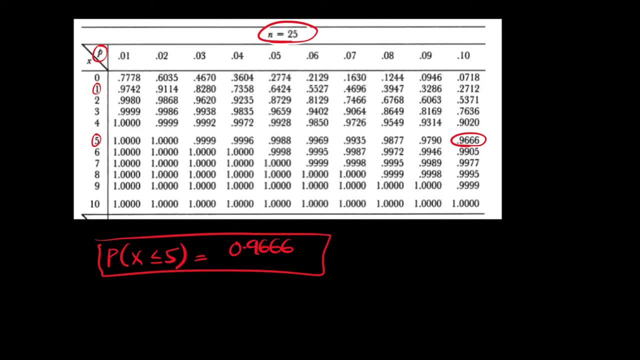 answer for the problem. so this is how you can calculate directly from the table without having to calculate the value. so what if? if the value is given as such way that, if they give you p of x greater than or equal to 6, then what you would do here is you will take the total problem. so 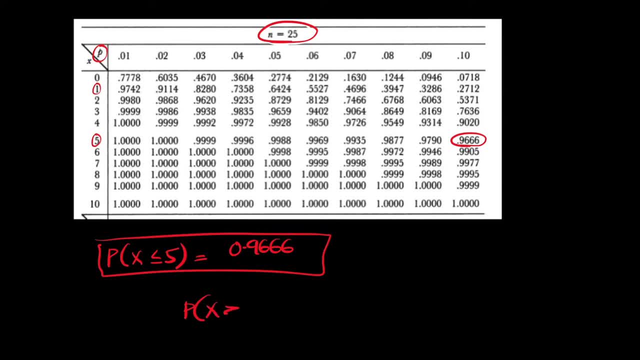 for example, let's say, if they ask you for p of x greater than 5, then you will take 1. the probability the formula is 1 minus p of x less than or equal to 5. so this is how this formula can be used when you have a greater than value, and this is the value that you have, so substitute it. 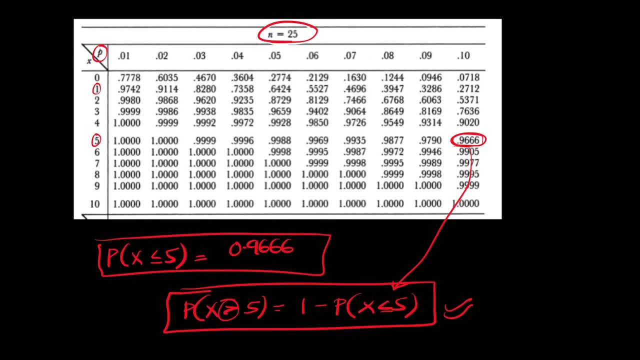 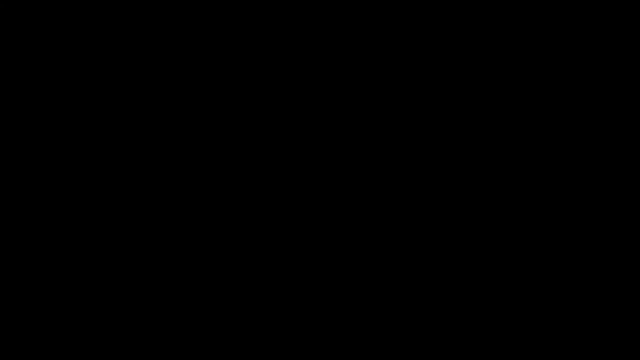 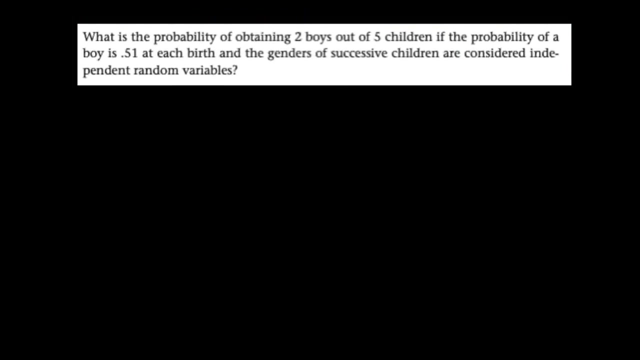 into this problem and find your answer. so this is how you can solve binomial problems using tables. so let me give you some smaller examples so that you can solve directly. so let's say we have a problem here. so the probability: what is the probability of two? 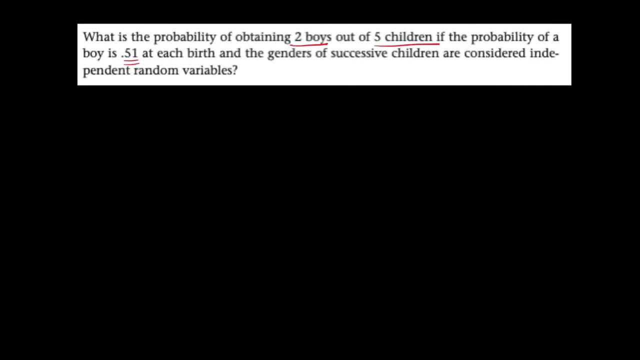 boys out of five children if the probability of the boy is 0.51 at each birth and the genders of successive children are considered independent, random variables. so here n is 5, x is 2, p is 0.51 and q is 0.49. so these are the values. they are asking you the probability. 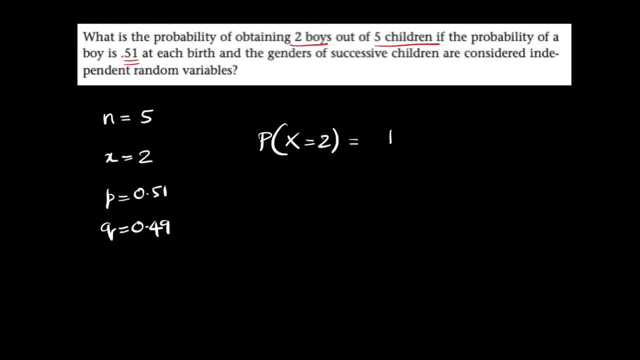 of two boys out of five children, so p of x equal to 2. again the formula ncx, p to the power, x, q to the power, n, minus x, so n, cx, n is 5, so 5, c, 2, p to the power, so p here is 0.51 to the power 2. and 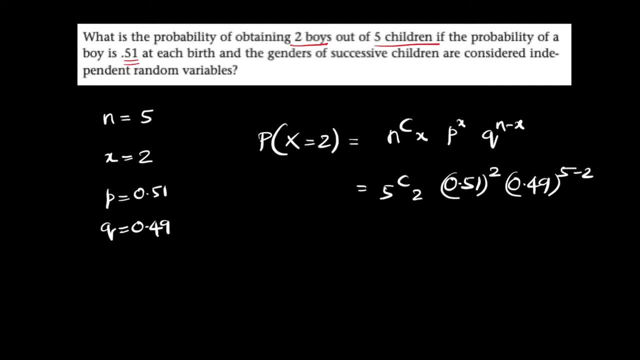 0.49 to the power 5 minus 2, so 5 c 2. so 0.51 to the power 2 and 0.49 to the power 5 minus 2. so how would you find the value for this? so 5 c 2, so this becomes 0.51 square. 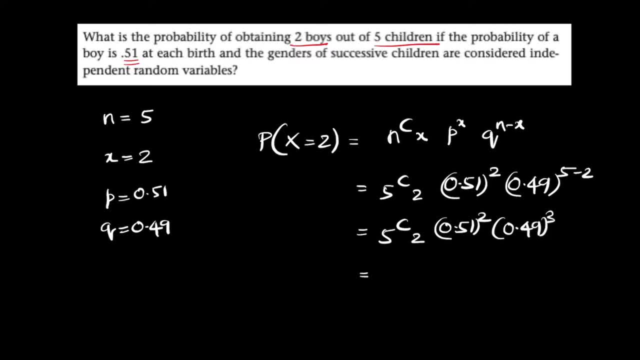 into 0.49 cube. so 5 c 2 is you can write it as 5 2, so you can replace this 5 c 2 as 5 2, so which means that write 5 factorial in reverse for two values, 5 times 4 by the down ones factorial. 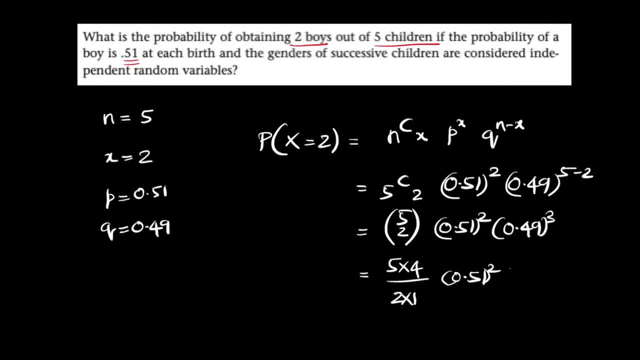 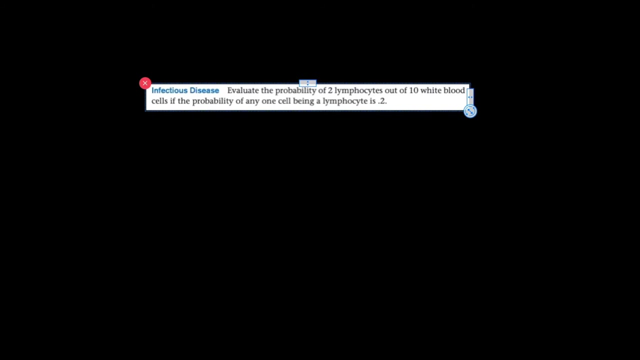 2 into 1 times 0.51, square into 0.49 cube. so use a calculator. so the value is 0.306. so this is the value for p of x equal to 2. so now you try another practice problem. so try this problem here. 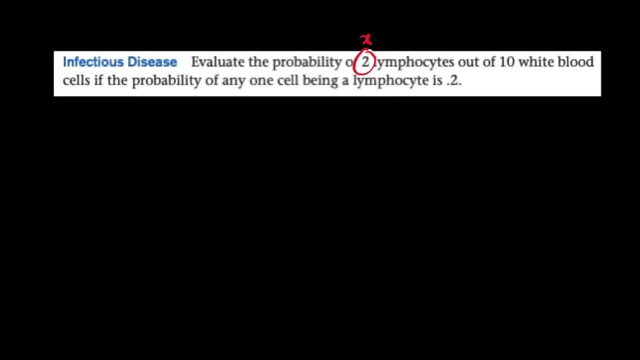 this value is x, 10 is n and 0.2 is the value of p. so x is 2, p is 0.2, n is 10. so obviously q is 1 minus p, that is 1 minus 0.2, so which is 0.8. so they: 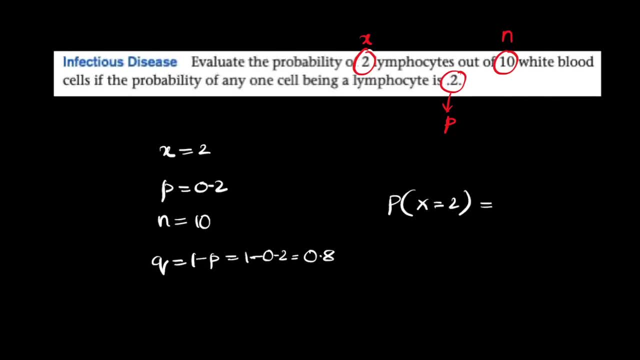 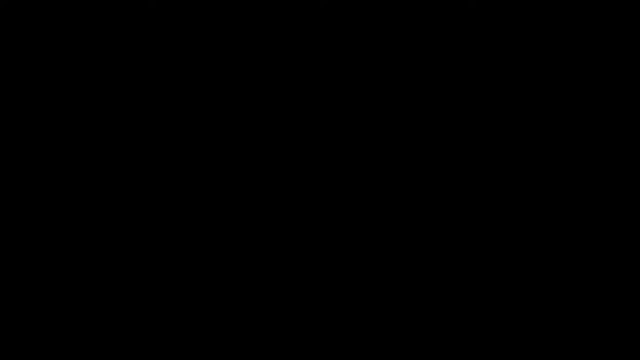 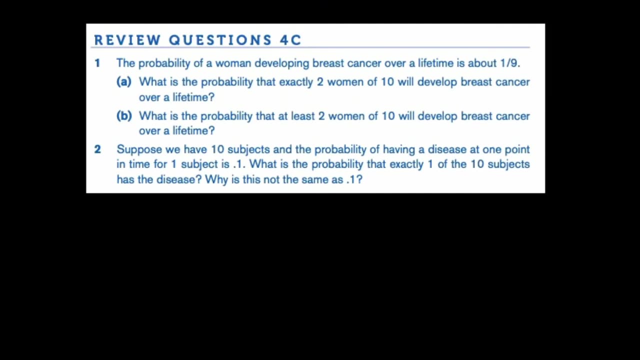 are asking you for the probability of x equal to 2. so pause the video right here and try to solve this problem. so also try some review problems. so try these problems and see if you can get the answer correctly. so pause the video right here and try to solve this problem. so next let's come. 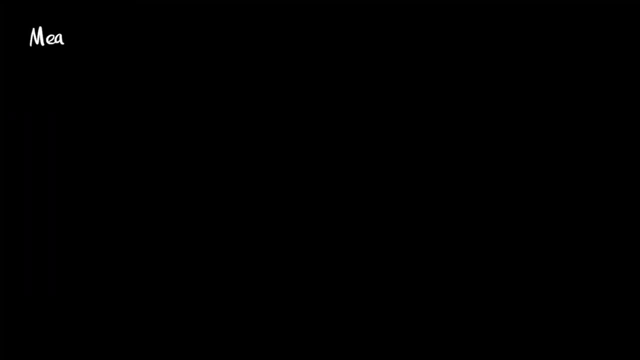 to the last topic of binomial distribution. the x, k minus powers are balls. so when we get a value y, we only have two types of eigenvalues and the rest of them have their eigenvalues b and c. this can be some common formations ofง ys, kind of something like yx k is equal to 1 and yx n- not always right. so instead 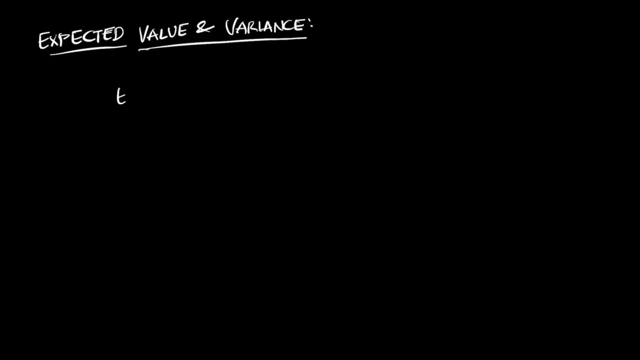 we are looking for a function where theaware force is equal to 1 and yx is equal to 1. so that is what it says. if we one more time ask this question, and after the production of the uniformed next expression, we can find that it gets to the value of p of x, that is. 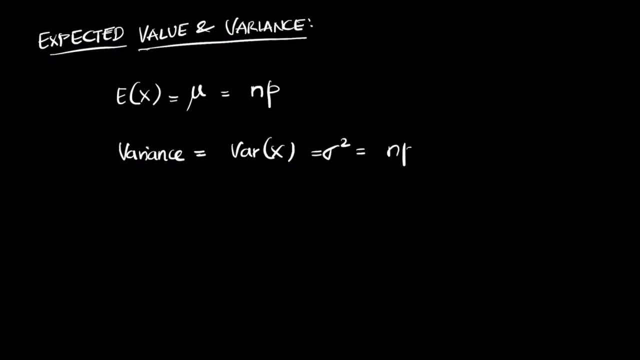 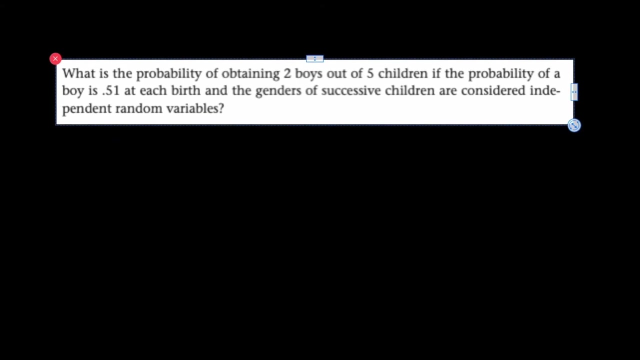 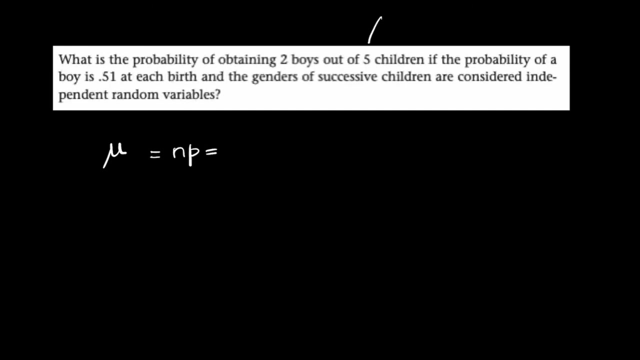 of x, or sigma square is npq. So mu here is np, sigma square is npq. So these are the two formulas that you can remember for the expected value and for the variance. So let us try a problem, So for this problem, so let us try and find the mean. So mean is np, n here is 5 and p. 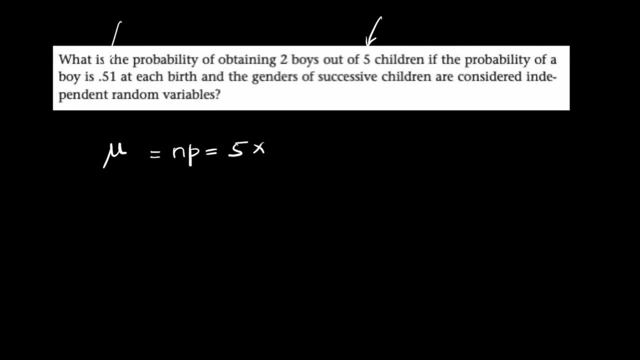 here is minus 2.. So let us try and find the mean. So let us try and find the mean. So let us try. here is 0.51. so n is 5 times 0.51. so when you calculate, 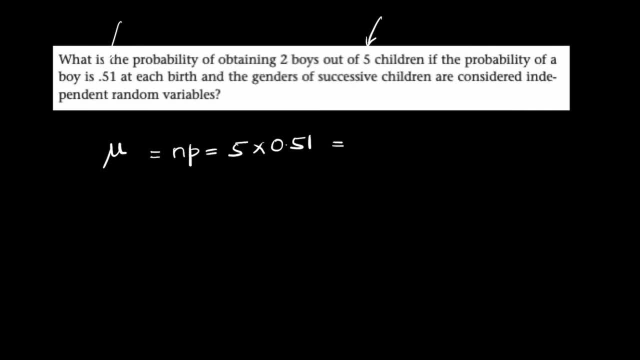 when you calculate 5 times 0.51, that gives you a value of 2.55. so the mean number of boys out of 5 children is 2.51, 55. so this is how you know the variance. so the mean so sigma square is: 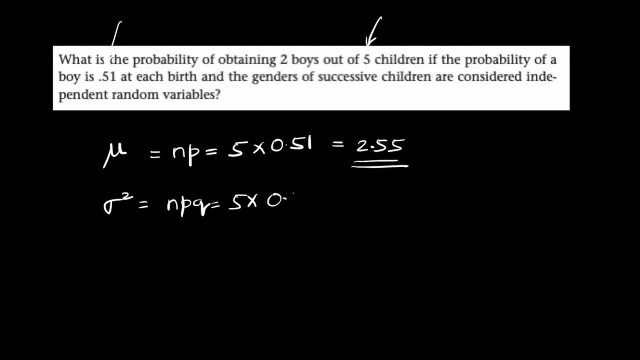 n, p, q. so n is 5 times p is 0.51, times q is 0.49. so just multiply the mean with 0.49. that gives you also the same answer. so that is 1.2495. so if you want to calculate sigma, so sigma becomes the. 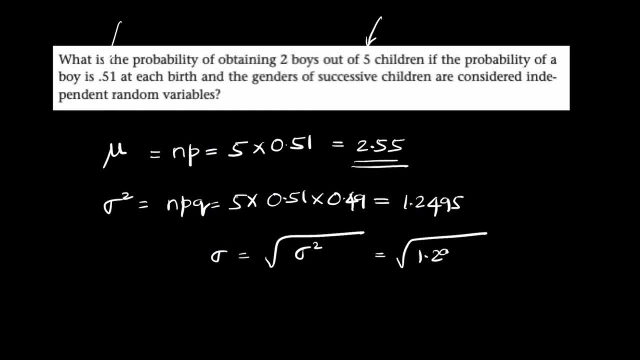 square root of sigma square, so square root of one point two, four, nine, five, so that value becomes 1.1178. so the variation, the standard deviation is 1.1178 boys. all right, so this is the mean and variance and the standard deviation in a binomial distribution. 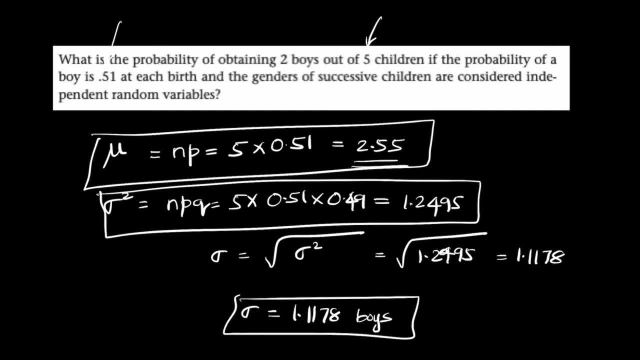 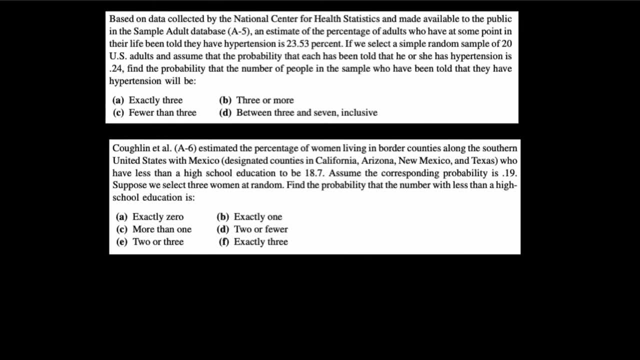 so with this we end binomial distribution. so try some practice problems for bernoulli's binomial distribution. and so pause the video right here and try to solve these two problems. note down the probability correctly, note down the sample size and try to do it on your own so that you get easy. you get acquainted to the data. 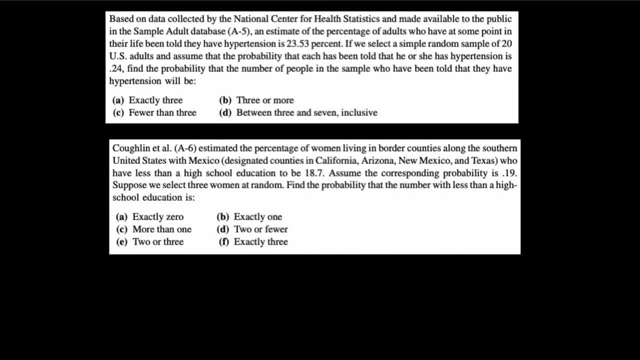 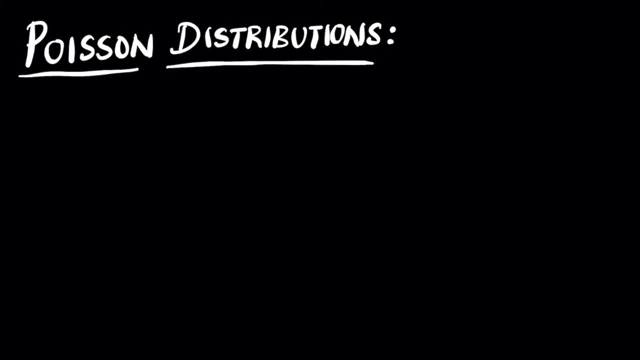 so pause the video right here and try to solve this problem. so let's discuss the last distribution and discrete ones: poison distribution. so poison distribution is generally used as a subsequent distribution for binomial distributions. when n is too large and p, the probability of success is too small. so these are the conditions. 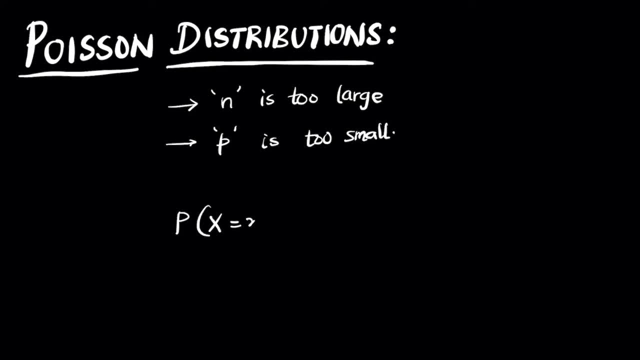 that we generally use it until so that it is defined as p of x equal to x. equal to a power negative lambda times lambda power, x by lambda factor, x, factorial. so where x is either 0, 1, 2 and so on. so here x is the desired event. 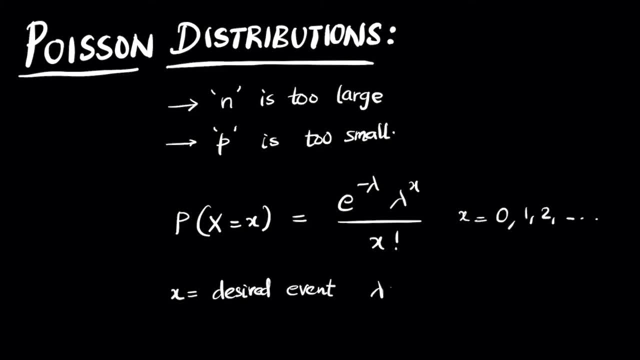 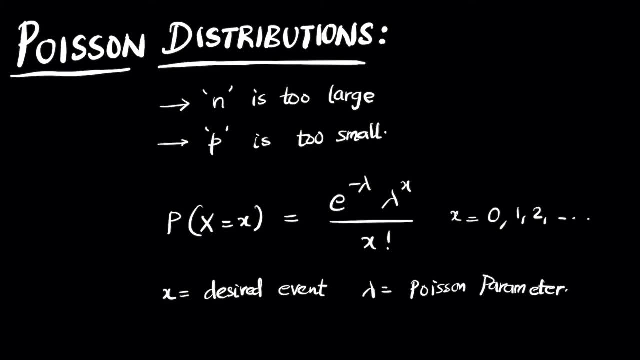 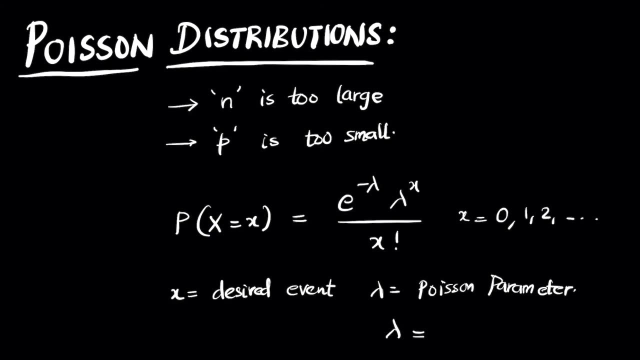 lambda is called as the poison parameter, right? so lambda here is called as the poison parameter. so most common way for calculating lambda is the same lambda here the peculiarity of lambda is that it is a Poisson parameter and it is a Poisson parameter so it can be used as both mean and variance of the poison distribution. so it can be used as both mean and variance of the poison distribution. 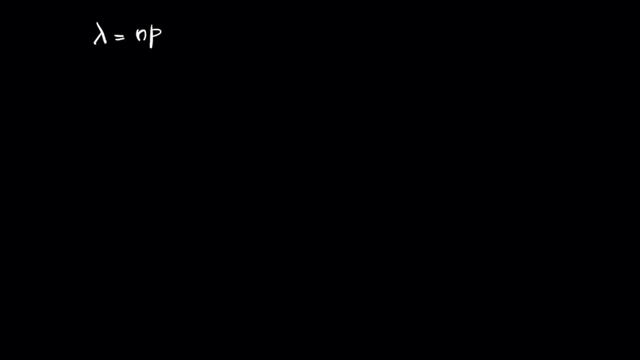 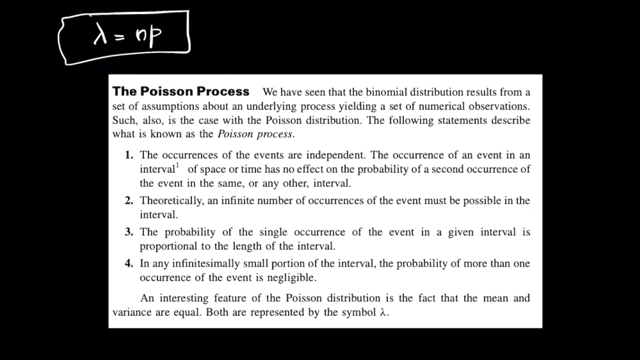 so generally, lambda is calculated as np, as an approximation from the binomial distribution. so what is the poison process then? so there are certain assumptions that we have to consider. so the following statements generally describe the poison, clear, clearly, the poison process. so, number one, the occurrences of events are independent and 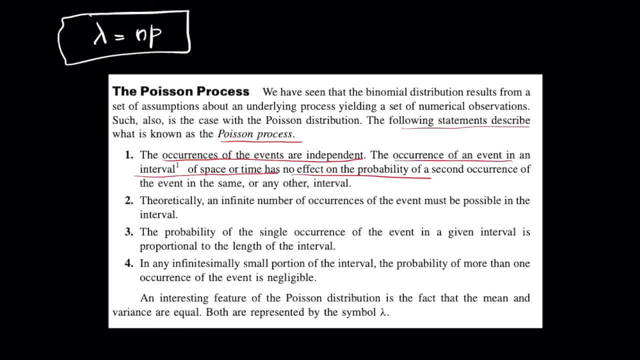 the occurrence of event in an interval of space or time has no effect on the probability of second in the space or time. so, theoretically, an infinite number of occurrences of the event must be possible in a given interval. notice that the number of events possible are infinite and the probability of single occurrence is proportional to the length of the interval. 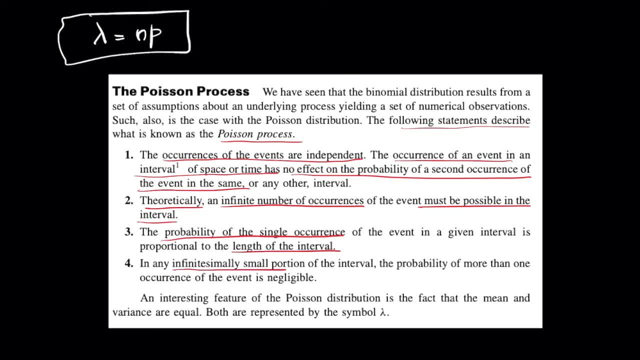 meaning that it's really small. so in an infinitesimally small portion of the interval the probability of more than one occurrence even is negligible. so when you have more than one event that's nearly not tangible. so the interesting feature of poison is that both mean and variance are equal and they're also represented by the parameter. 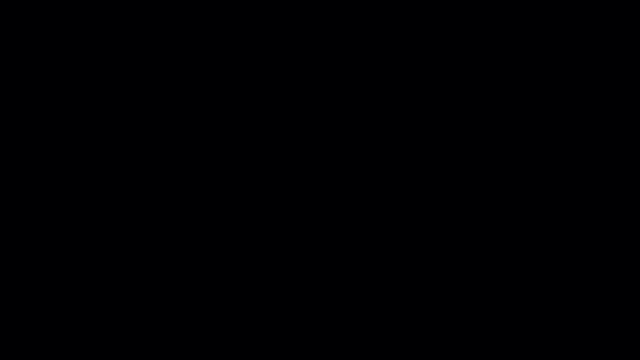 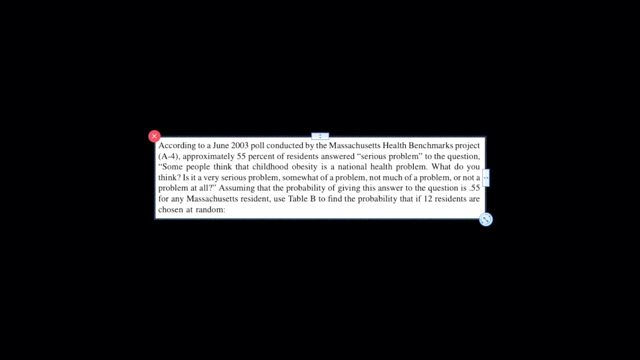 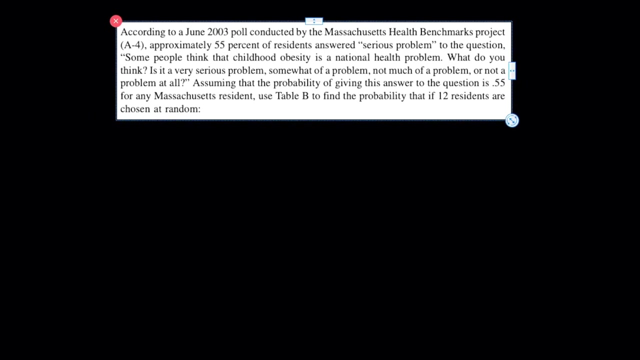 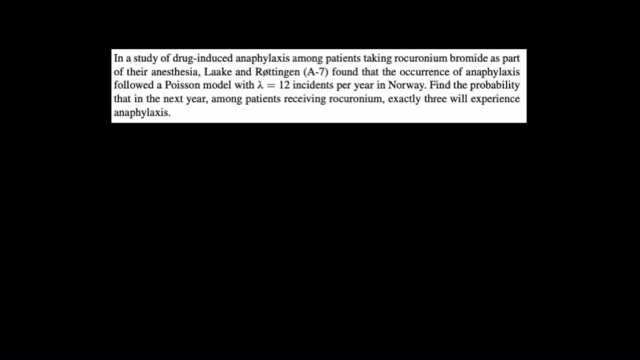 the parameter, the lambda parameter. so let's try some problems and let's try and understand how poison distribution works. poison distribution Kubacki. so let's try this problem. notice that in this problem lambda value is already given and they are asking you to find the probability. 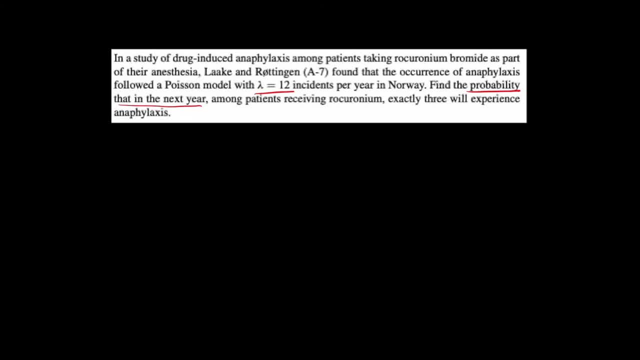 that in the next year, among patients recovering rocanorium, exactly three will experience anaphylaxis. so here, lambda, is 12 e x. here is what you want is exactly 3, p of x equal to. so they are asking you to find p of x equal to 3. so we know the formula e: power negative lambda. 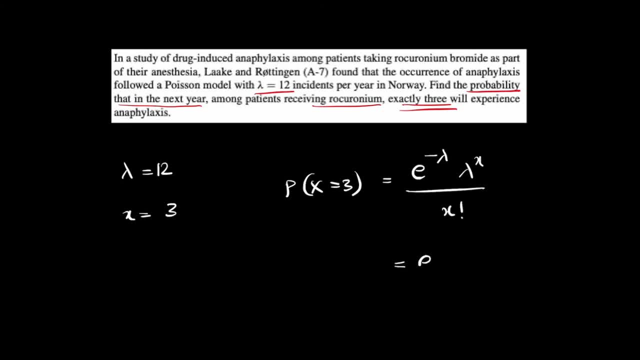 lambda power x by x factorial, so e power negative lambda is negative. 12 into 12. power 3 by 3 factorial, so e to the power negative 12 times 12 cube by 3 factorial. so when you calculate the value that you is 0.00177. so this is the probability that at least three patients will experience anaphylaxis. 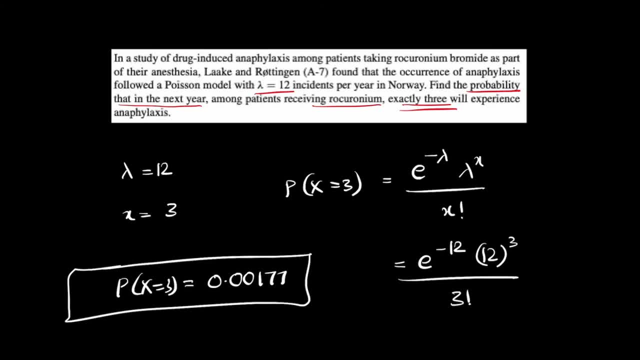 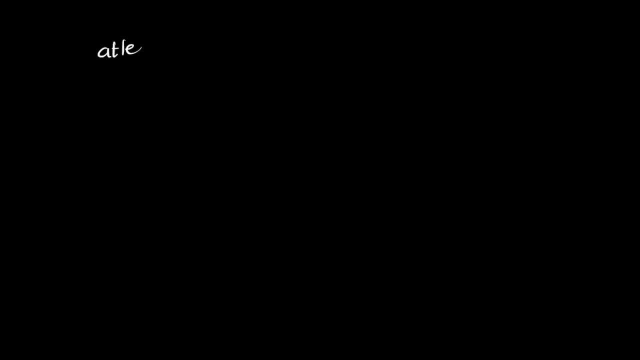 so what if the question says the exact same question and if it says at least three? how would you find it so at least three? we know that it's greater than or equal to three. so the entire probability sum is one. so we know that p of x greater than three can be written as: 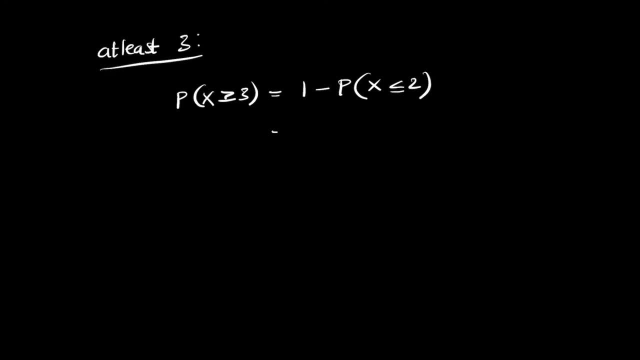 1 minus p of x less than or equal to two. so which means that one minus of p of x equal to one. zero plus p of x equal to one, plus p of x, equal to two. so remember that we are not going to find greater than or. 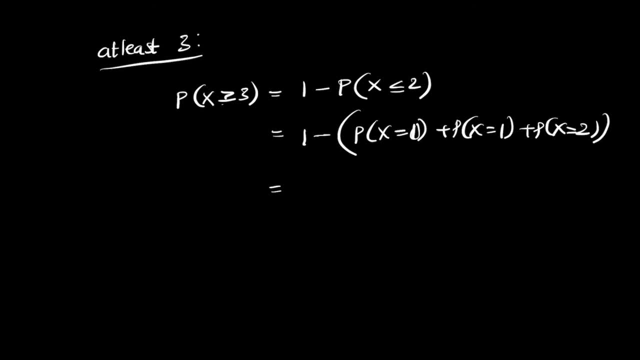 equal to three, because there are infinite number of events. so we can simplify this and write it down like this way. so the formula becomes now: p of x equal to zero is e power negative lambda into lambda power zero, so lambda. here is 12. so e power negative 12 into 12 power negative lambda. 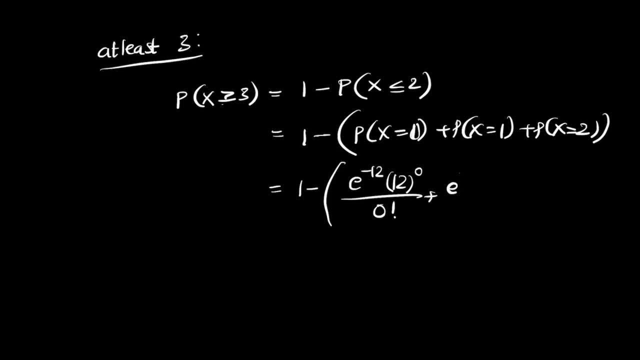 into 12. power 0 by 0, factorial plus e power negative 12 into 12. power 1 by 1 factorial plus e power negative 12 into 12 square by 2 factorial, so 1 minus the values are, so the entire sum is: 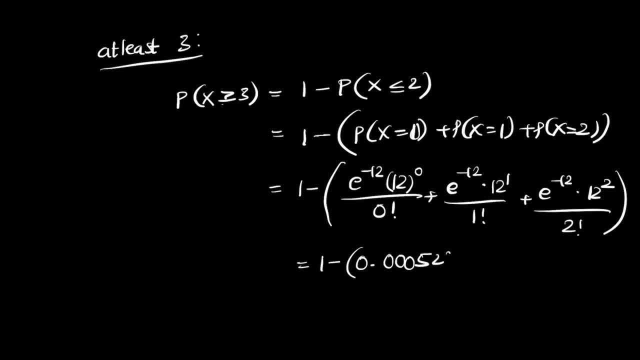 going to be zero point. triple zero phi, triple two phi. so that becomes zero point. triple nine four, triple seven, five. so this is the probability of x greater than or equal to three. so whenever you want to find the formula, remember this: x greater than or equal to x. 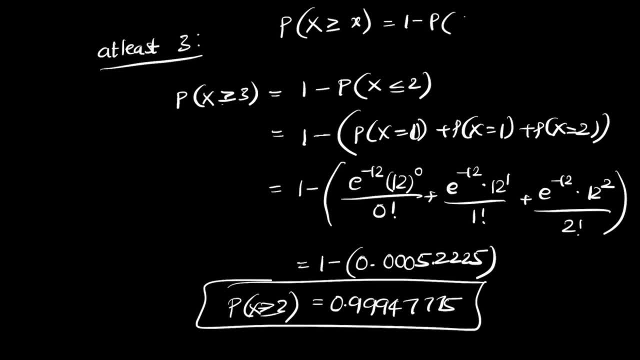 is 1 minus p of x, less than or equal to x minus 1. so this is the formula that you can use when you have greater than or equal to. if you have less than or equal to, you can directly take the sum. for example, in this, in this problem, if you have greater than or equal to x, greater than or equal to, 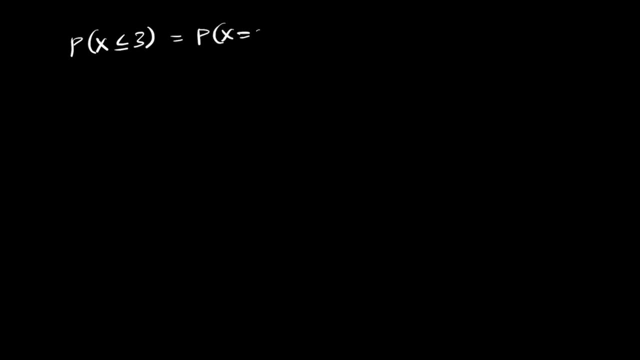 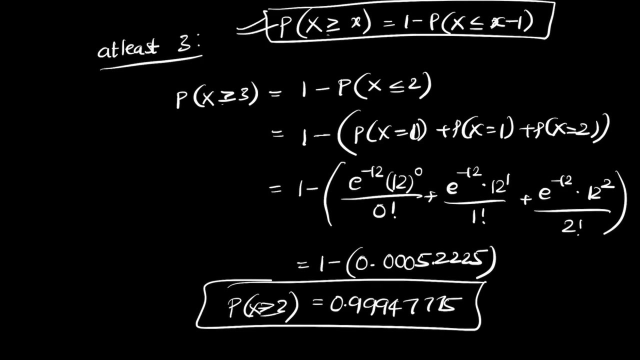 x less than or equal to 3, then you would have directly calculated x equal to 0 plus x equal to 1 plus x equal to 2 plus x equal to 3 to make it easier. but because it is greater than or equal to we have, we will have to change the formula and try to find it in an easier manner. so this is: 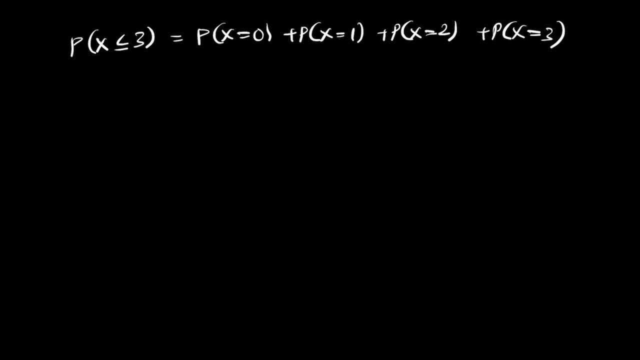 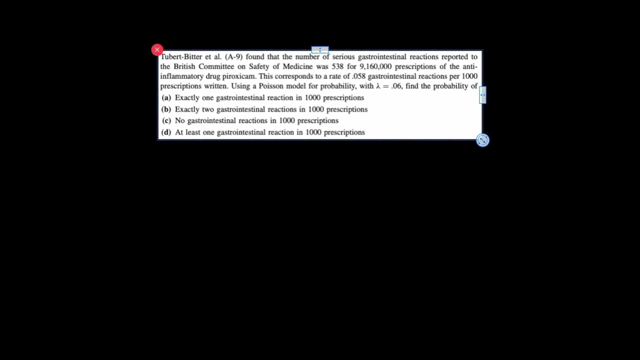 poison distribution. now, in a poison distribution, the expected value and variance, all e of x is lambda. sigma square is also lambda. so remember that both the values are the same. so let me give, let me give you some more problems for you to practice. so here everything is given, lambda is given, so they. 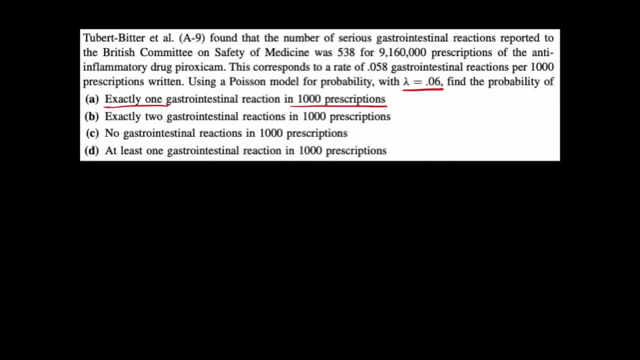 are asking exactly one in one thousand prescriptions, and next is exactly two in one thousand prescriptions: no gastrointestinal reactions in one thousand. so here you have lambda, which is 0.06, and n, which is thousand, and they are asking you to find, for the first one p of x equal to 1, in the second one p of. 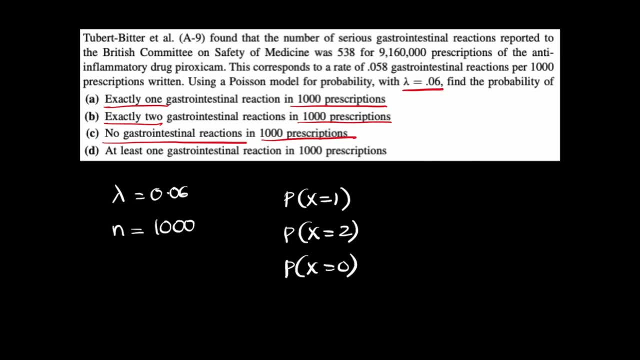 x equal to 2, in the third one p of x equal to 0, and the last one is p of x less than or equal to 1. so for the last one it should become x equal to 0 plus x equal to 1, so you already have x equal to 0 and x equal to 1. when you find the 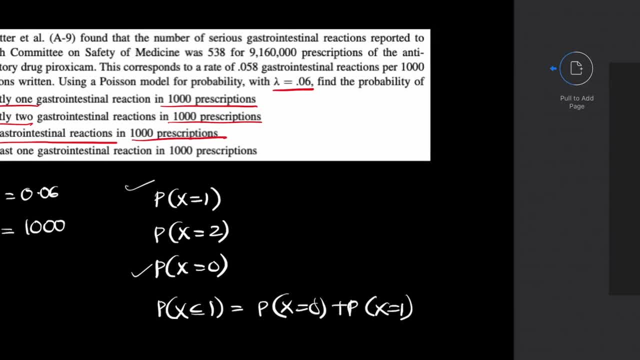 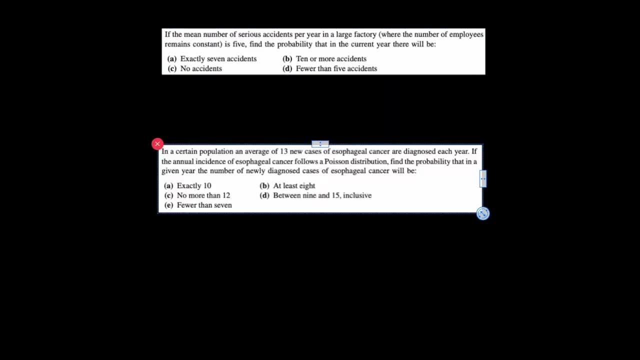 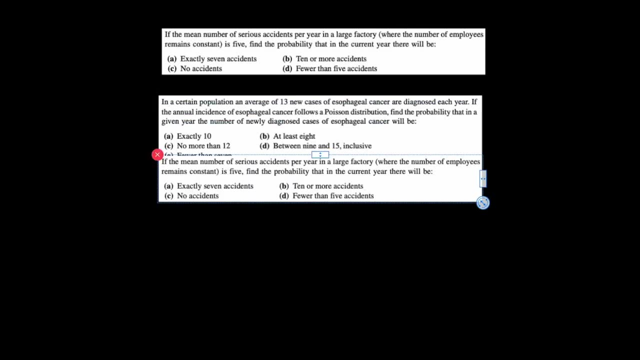